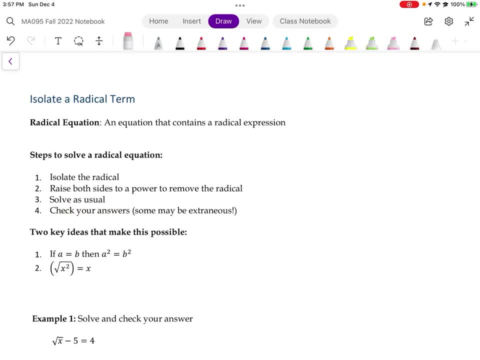 All right. so two key ideas that make this possible: If a equals b, then a squared equals b squared. The square root of x squared is x. The square root of x cubed, the cube root of x cubed is x. right. The cube root of x cubed is x, and so on. and 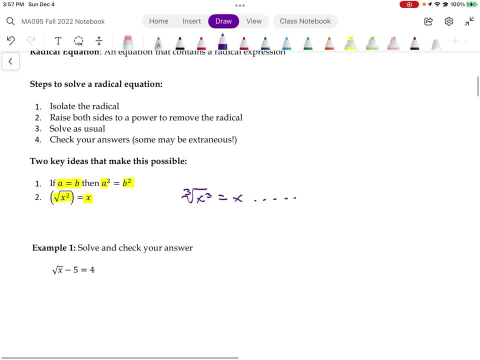 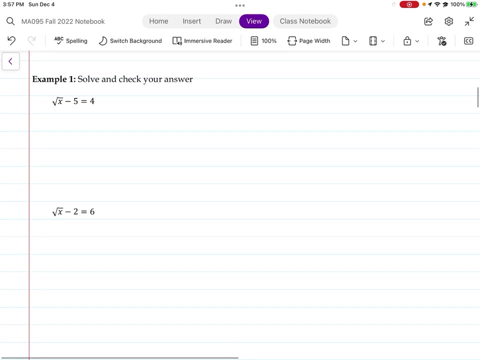 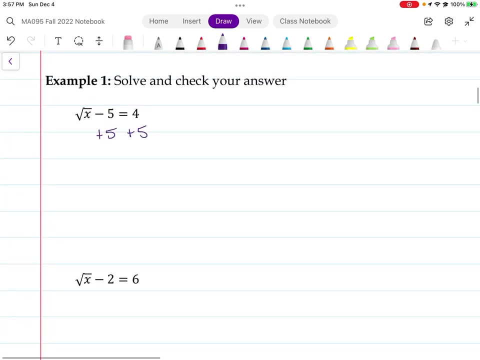 so on. All right, so solve this and check your answer. All right, and I would like some lines, So I'm going to go add some lines here. All right, so we've got, we've got to add the 5 to both sides first. So we're going to add 5 to both sides And I 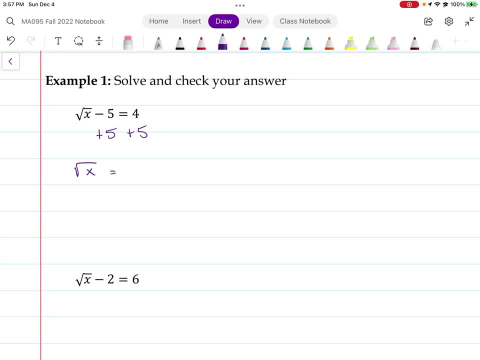 get the square root of x equals the 5's go away on the left and I get the square root of x equals 9.. So I'm going to square both sides. So I'm going to do this and I get a. 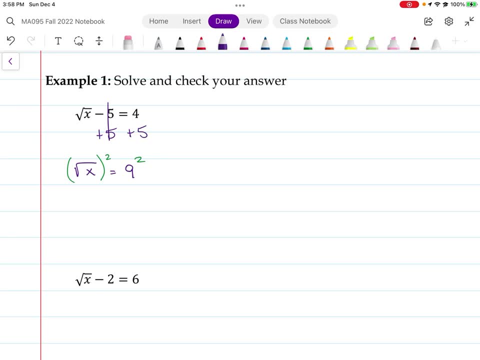 square root of x squared. square root of x squared is x, 9 squared is 81.. So check means to really check, because we're going to get to some that really you will get answers that don't work. It looks like this: So the square root of 81 is 9 minus 5 is 4.. Is that? 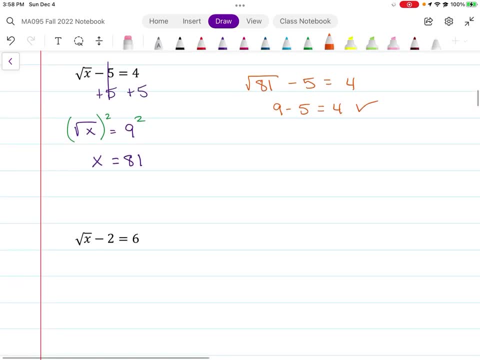 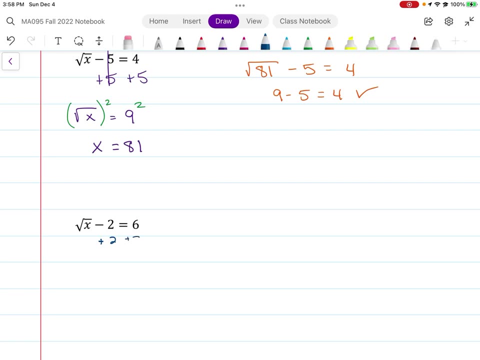 true, Yes, it is All right. so give this one a try. the second one: All right, so we're going to add 2 to both sides, And by both sides I mean the equal sign. Both sides have the equal sign, All right, so I get square root of x, These 2's. 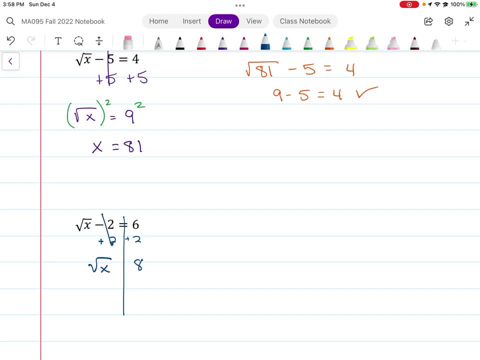 become 0, and I get 6 plus 2 equals 8.. Now I have to square both sides And I'm going to get that x equals 64.. Okay, x equals 64.. So let's check it: Square root of 64 equals. 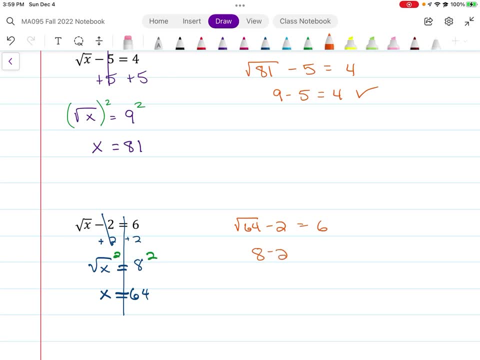 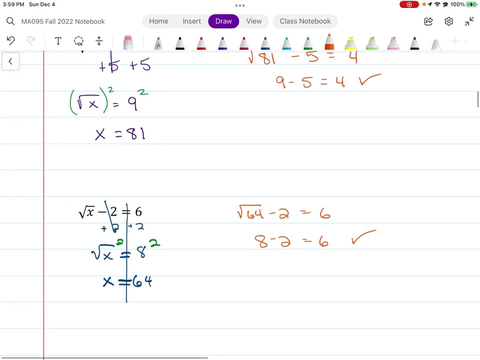 4 minus 2 equals 6.. 8 minus 2 equals 6.. Yes, All right. so remember, when we do these, we are only looking at the principal root, We're not looking at the negative, and it has to do with the fact that the negatives can't be included because it would make it. 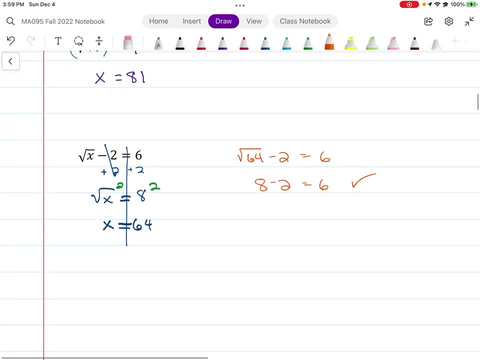 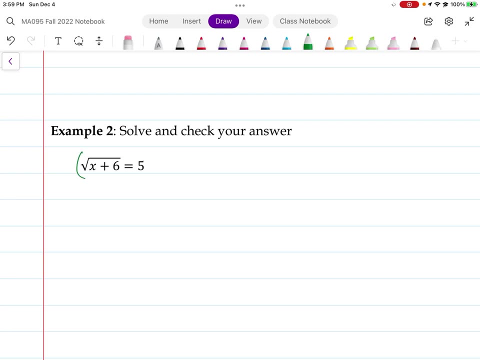 so that it is not a function and we're doing only functions. All right, so solve and then check your answer. So how would you solve this? Well, what you're going to do is just square this whole thing, And that means we have to square the other side. All right, so if I square that whole, 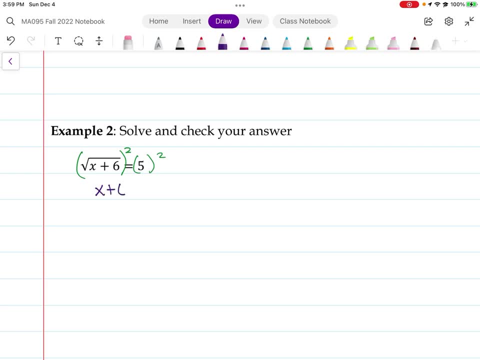 thing I get. x plus 6 equals 5, squared is 25.. So remember, when you square the whole thing, the whole x plus 6 had the square root go in there. So when we square it, the square root just goes away and we get x plus 6.. Now we're going to subtract 6 from both sides. 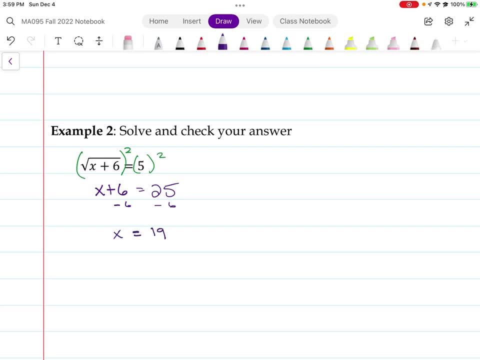 and I get that x equals 19.. All right, so let's check it, New orange, The square root of 19 plus 6 equals 5.. The square root of 25 equals 5? Yes, that's true, All right. 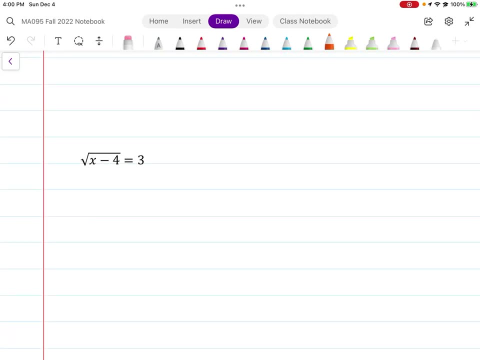 why don't you try this one? All right, so we're going to square both sides, the whole thing, And so we get x minus 4 equals 9.. Add 5, 4 to both sides and I get x equals 13.. 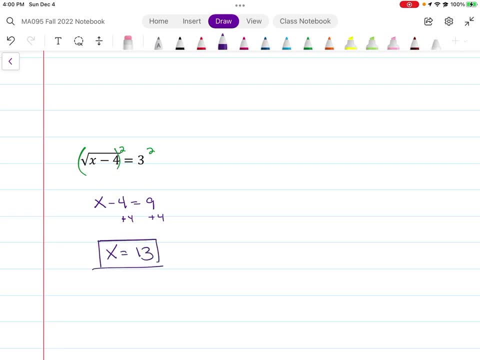 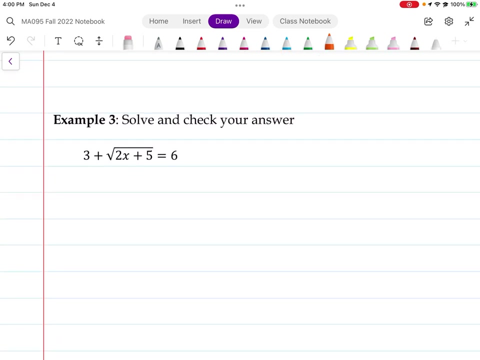 That's the answer, but let's check it. So we get: square root of 13 minus 4 equals 3.. The square root of 9 equals 3.. Yes, that checks All right. continuing on Another kind of problem, We've seen problems similar to this with some other kinds of functions besides. 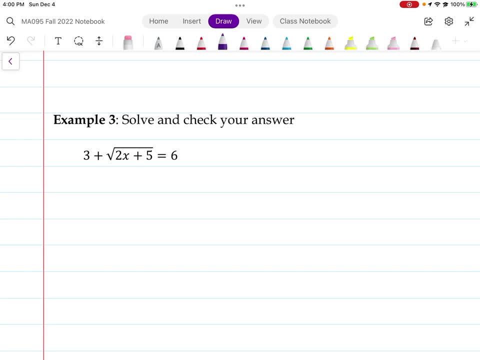 square roots. All right. so we need to isolate the square root so that we can square both sides. If we squared it right now, we'd end up with a mess because we would have to FOIL the left side. We don't want to do that right. 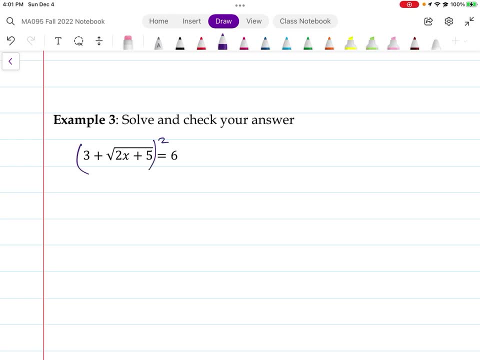 If we squared this, we would have to FOIL it, because we'd have 3 plus the square root of 2x plus 5 and another 3 plus the square root of 2x plus 5. And that would be a mess. 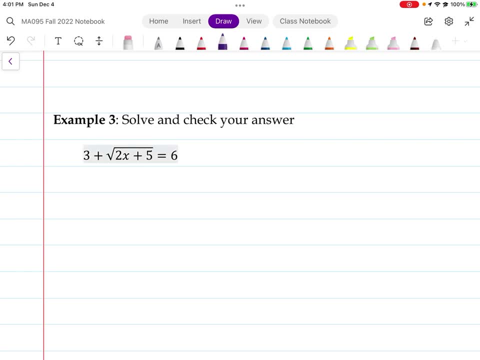 so we're not going to do that. We're going to first isolate by subtracting 3 from both sides, And I get the square root of 2x plus 5 equals 3.. All right, now we can square both sides. I square a square root. 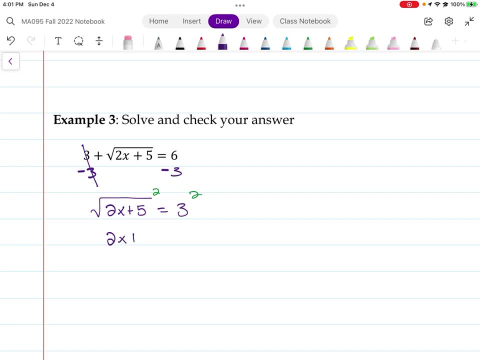 13 plus 12 equals 3.. So that's the square root of 2x plus 5.. All right, now we can square both sides. If I square a square root, it just kind of cancels it out and I'm left with what's inside. 2x plus 5 equals 9 all. 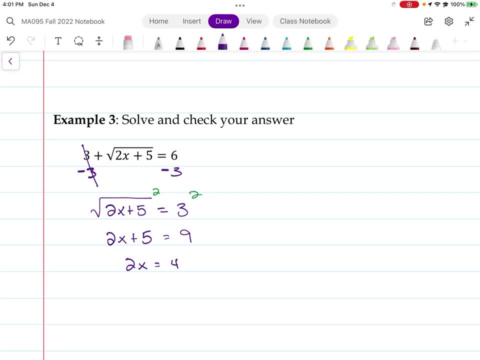 right. subtract 5 from both sides and I get 2x equals 4 divided by 2, and I get x equals 2. so let's check. I encourage you to pause the video and check these yourself so you can get used to doing it. 2 times: 2 plus 5 equals 6, 3 plus 4 plus. 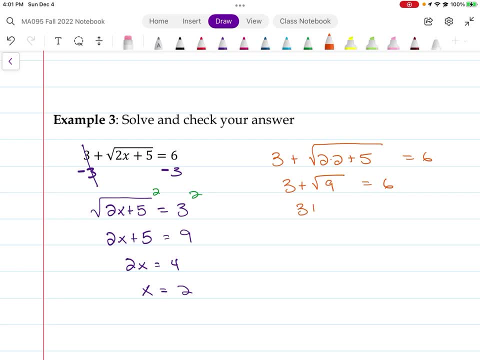 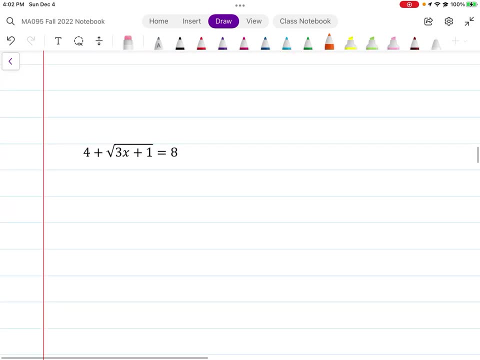 5 squared a 9 equals 6. 3 plus 3 equals 6. that checks. all right, give this one a try. all right, so you subtract 4 from both sides and you're left with square root of 3x plus 1 equals 4. now we're going to square both sides and we're left with 3x. 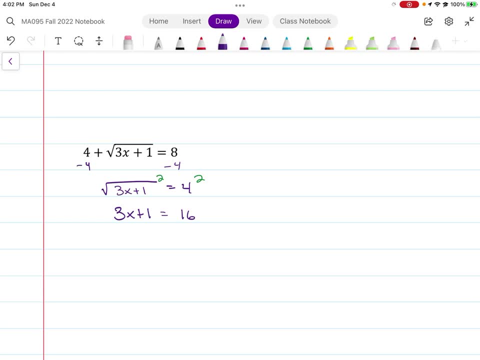 plus 1 on the left equals 16.. Subtract 1 from both sides, I get 3x equals 15.. Divide by 3 and I get x equals 5.. Now, if you checked it, you would get 4 plus the square root of 3 times. 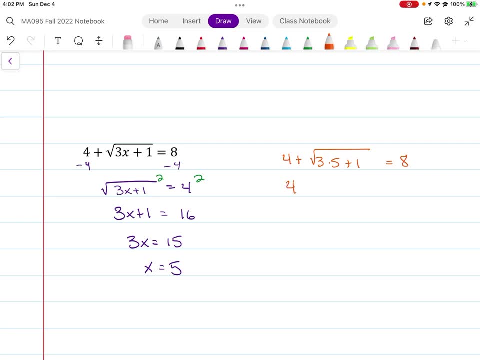 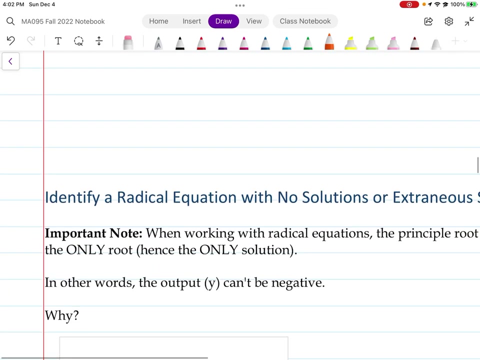 5 plus 1 equals 8.. 4 plus 3 times 5 is 15 plus 1 is 16. so the square root of 16 equals 8.. 4 plus 4 equals 8. yes, Okay, identify a radical equation with no solutions or extraneous. 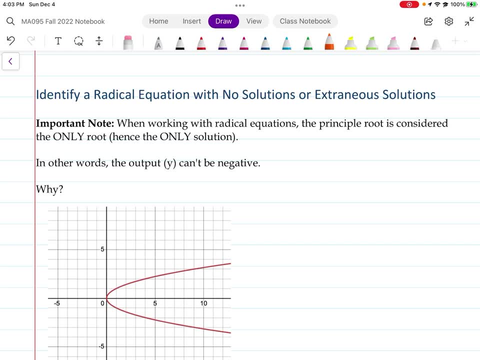 solutions. So this is where it gets kind of challenging, because you have to kind of take one extra step, really thinking about your answer and does it make sense and why and why not? So an important note is: when working with radical equations, the principal root is considered the. 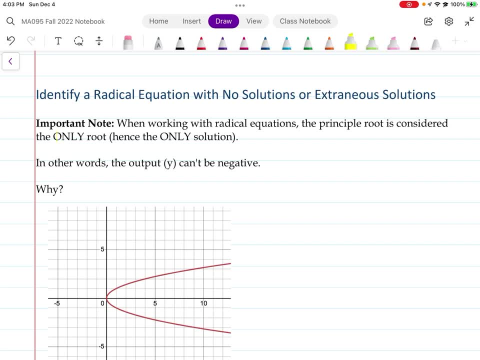 only root, root- and I said that just a moment ago, but now I've written it down- the only root, the principal root, that means the positive one. hence it's the only solution. in other words, the output Y can't be negative. and why is that? I want. 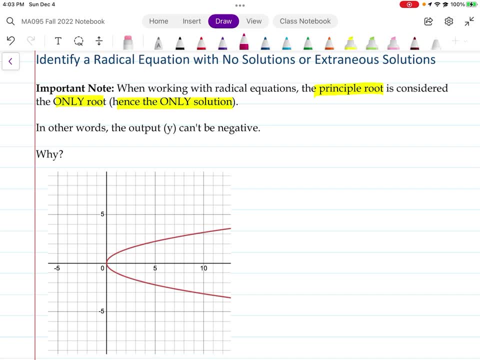 you to look at this picture of this. this is a. this is X. Y equals X squared. that would be what it looked like if you've graphed both the positives and the negatives, if you accepted negatives and positives there. so if you got a Y when you squared it and you took the square root and you took the negative answer. 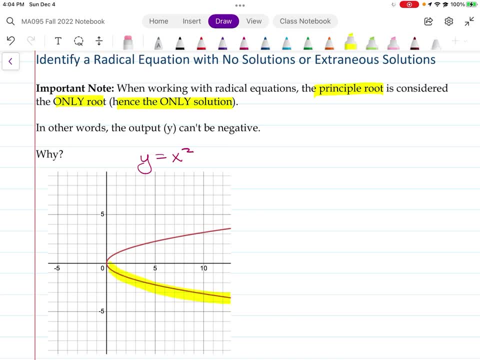 you would end up with these down here. it's the best way I have to explain it. this is a hard one to explain. so is this a function? no, it does not pass the vertical line test right. so what we do is we say: well you, you get the square root and you took the negative answer and you're going to 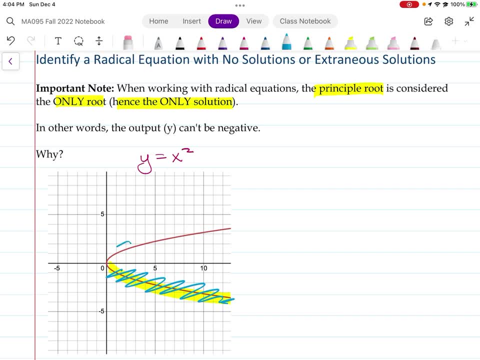 we're just not going to look at that half, we're only. we've chosen to do the positives. it makes life easier. why? who wants to do all negatives? as the answers right, so we got to do one or the other. so we have. all the mathematicians in the world have decided that the principal root is going. 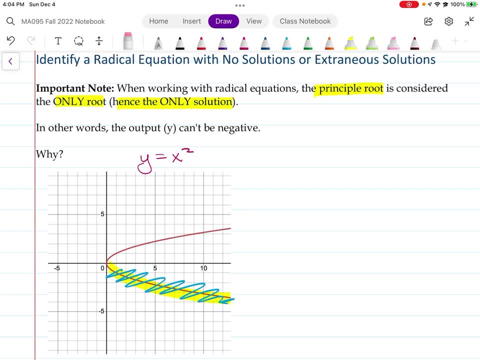 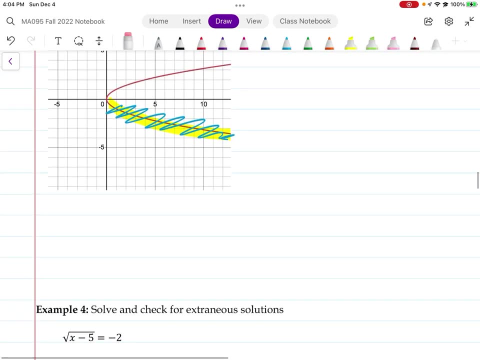 to be the positive one, the upper half. now it is a function. it passes the vertical line test if we don't include the negative answers. okay, so that's why. all right, so solve and check for extraneous solutions. so what we're going to do here is we're going to square both sides, and don't forget to. 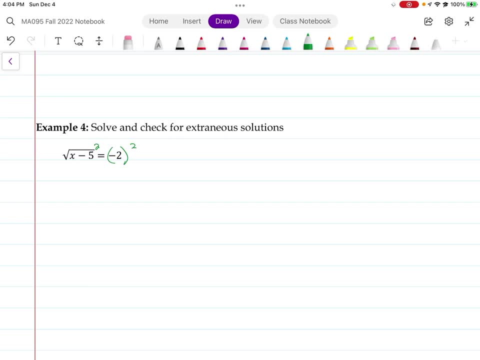 square it like that, all right. so we get x minus 5 equals 4, so add 5 to both sides and we get x equals 9, all right, so now let's check, and this is where you do really have to check: 9 minus 5. 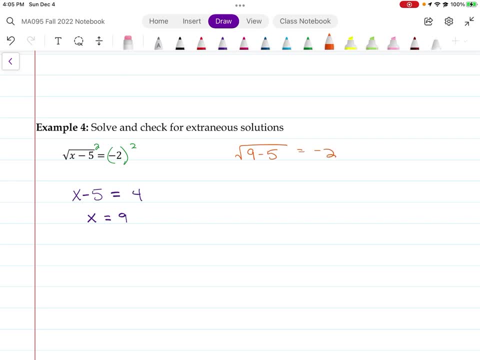 square root equals negative 2. the square root of 4 equals 9 minus 5. square root of 4 equals negative 2 and because it's a function, we're having to call this a function. now we're going to say, no, this is not true. this is not true because we are only doing principal roots. okay, so this is not true. 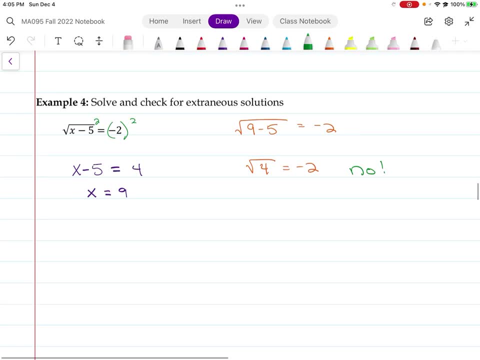 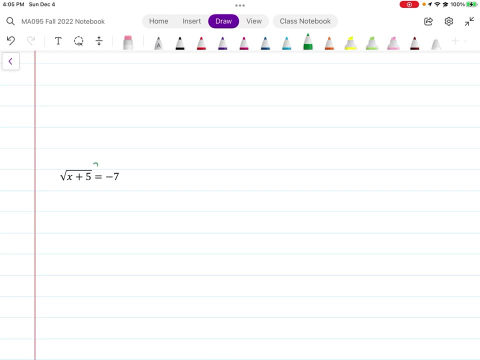 that is. that is, there's no solution to this, all right, why don't you try this one? all right. so if you square both sides, you end up with x plus 5 equals 4, and remember, we're squaring the whole negative 7, so it's a positive 49, so we're going to subtract. 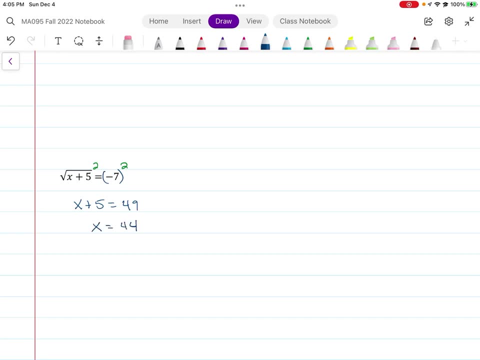 5 from both sides and we get x equals 44. now if we go to plug that back in, we get 44 plus 5. square root equals negative 7. the square root of 49 equals negative 7. no, the square root of 49. 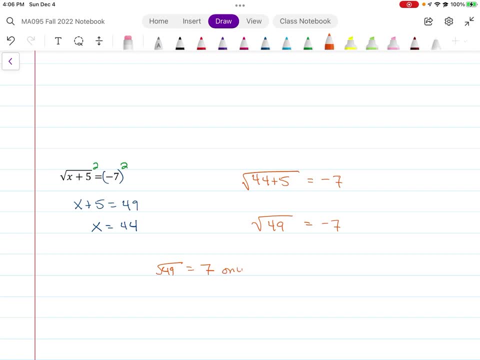 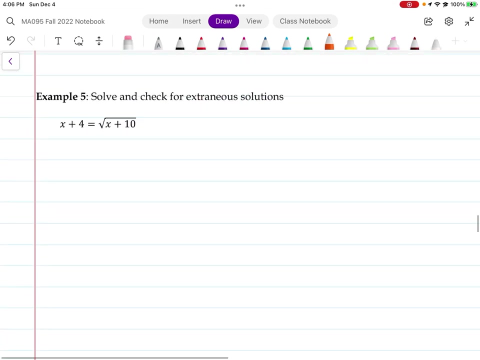 equals 7, only, only the only, the principal root. so no, there's no solution. all right, so solve and check for extraneous solutions. all right, so x plus 4 equals x plus 10, square root of x plus 10. so we're going to square both. 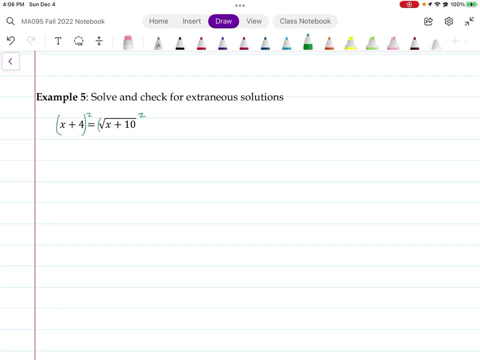 sides. that means we need to square the whole thing like that: square the whole thing so we get x squared plus 8x plus 16 equals x plus 10. all right, so subtract, and then we're going to solve using factoring. so we've got x squared. 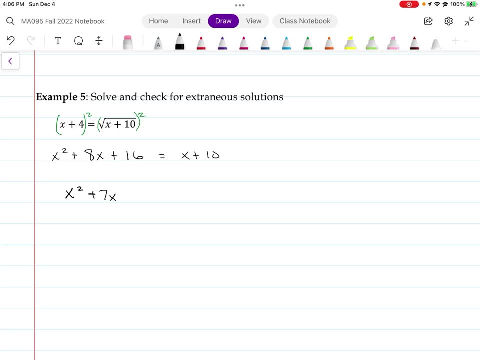 minus sorry, plus 7, x, um plus 6 equals zero. so i just subtracted x and 10 from both sides to bring it over to the left, and so it's equal to zero. i can only factor and solve when it equals zero, so i'm going to factor x plus six and x plus one. 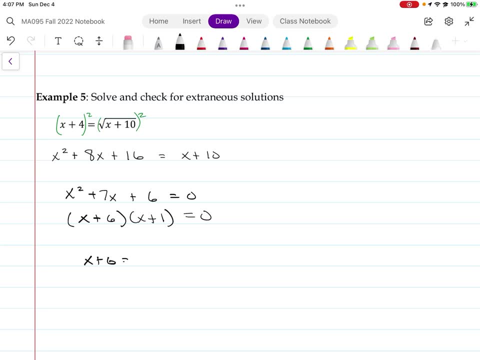 equals 0. So now x plus 6 equals 0 and x plus 1 equals 0, and we get x equals negative 6 and x equals negative 1.. Well, one of these is not going to work. There is only one solution to. 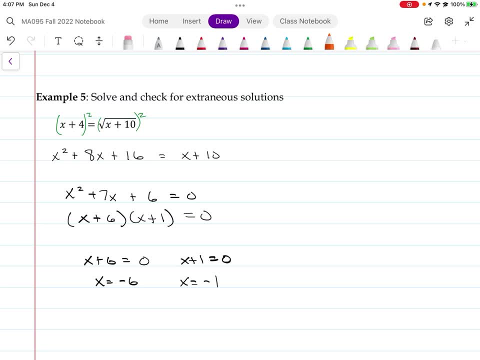 this one. That's my hint. So we're going to check both. All right, so we're going to check negative. 1 plus 4 equals the square root. So this is where x equals negative 1.. That's what I'm checking first: Negative 1 plus 10.. So 3: 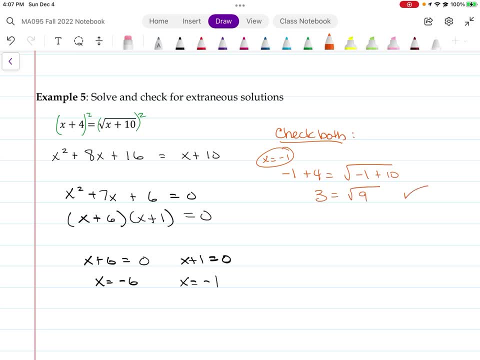 equals the square root of 9, and that is true. Let's try the other one: Negative 6 plus 4 equals the square root of negative 6 plus 10.. So this is where x equals negative 6.. All right, so we've got negative 2. 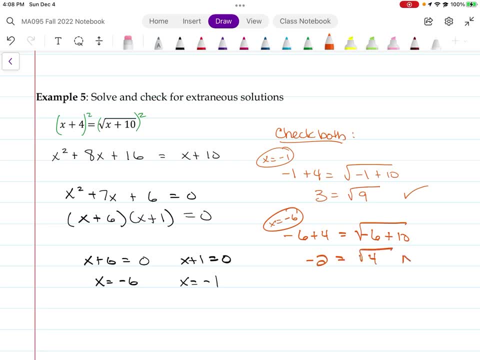 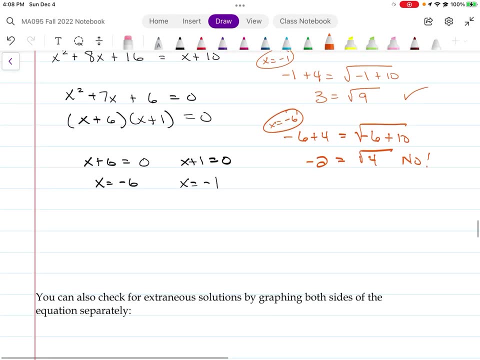 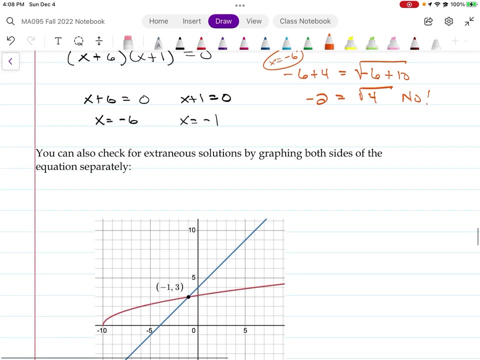 equals the square root of 4, and that is not true. No, because it has to be positive. All right, you can also check for extraneous solutions to something like what we just did by graphing. Okay, so we had two equations. We had x plus 4.. That's this blue one right here. 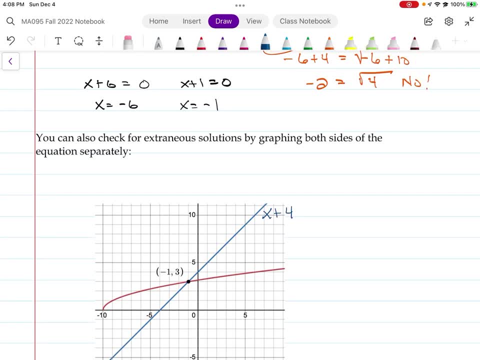 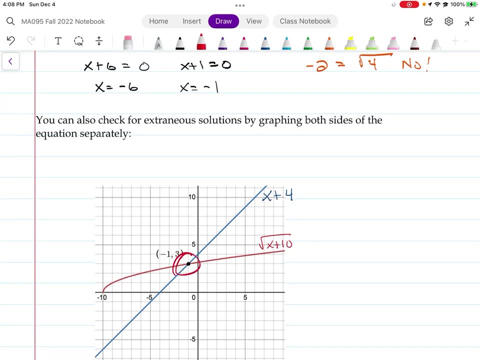 and we set it equal to the square root of x plus 10.. Square root of x plus 10.. That's this one. So I set this up ahead of time. There is one solution. It is right here. Well, where was the other solution? It's where they cross, It's where the two 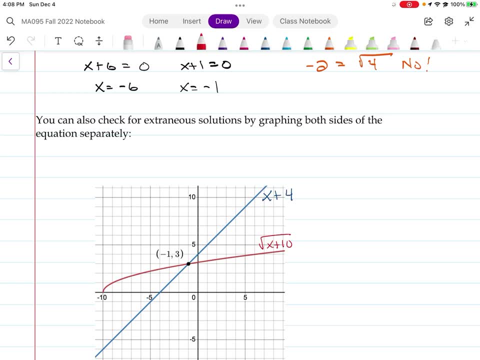 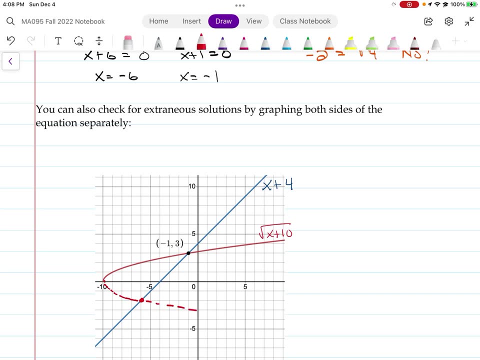 lines cross Two graphs. I should say So. the other solution was at negative 6.. Where's that? Well, that would have been this one right here. If the graph was allowed to come down here, that would have been the other solution. 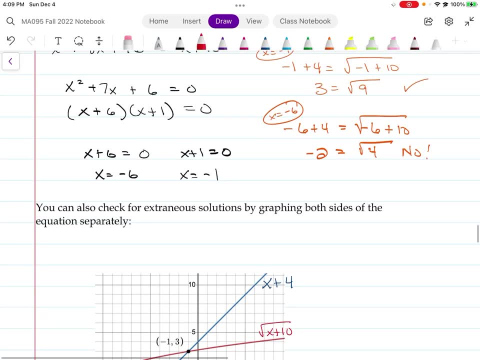 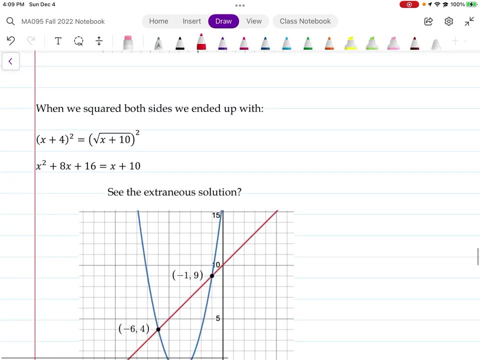 But we don't do that, So that's why that solution is negative. That solution is a no Okay, two different ways to think about it. All right. another way to think about it is: when we squared both sides, we ended up with these two different equations. Now, if 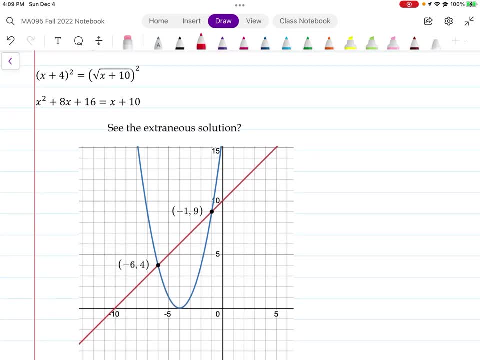 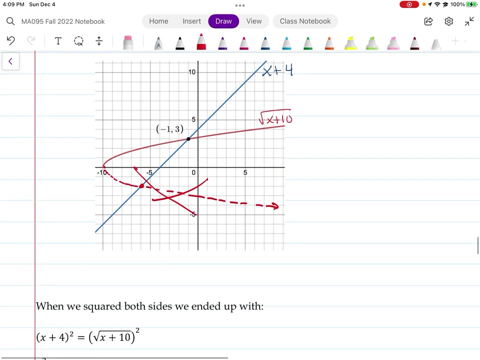 you square them and graph them. they look like that and they do have two places where they, where they touch. But this is the extraneous solution right here. That one's the extraneous one And the original equation it doesn't even. it doesn't exist. 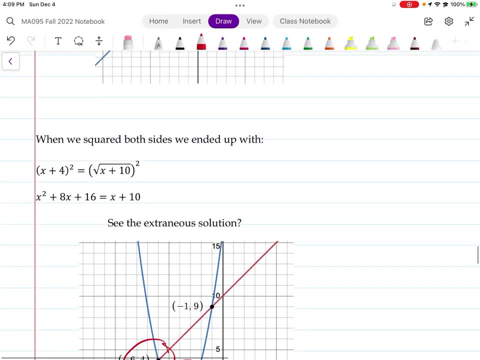 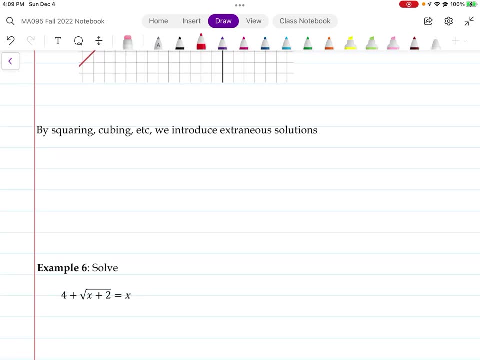 We don't use the half of the graph, Then it wouldn't be a function All right. so by squaring, cubing etc. we are going to introduce extraneous solutions, so you need to check for them. All right, we just have a couple more. 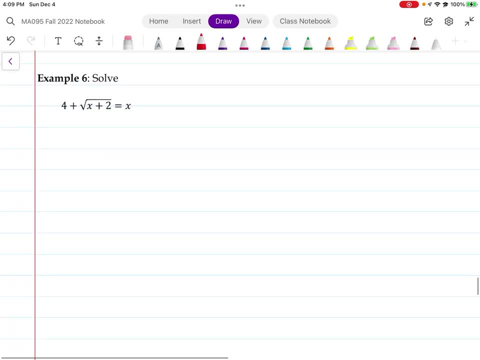 examples. Well, maybe more than a couple, All right, so solve this. How are we going to do that? Well, we're going to have to square both sides. The easiest way to do this is to subtract the 4. So the square root of the, the square root symbol, is: 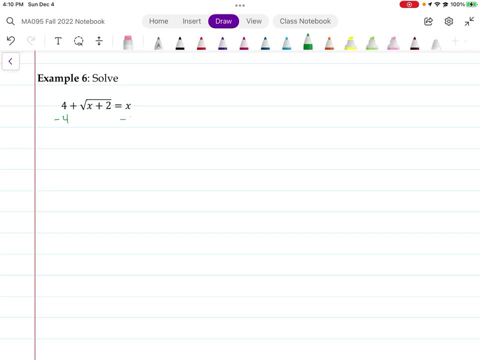 isolated, Just like we did with absolute values a while back. So we're going to subtract 4 from both sides and we get the square root of x plus 2 equals x minus 4.. So now we square both sides and we're going to get x plus 2 equals x squared minus 8x. 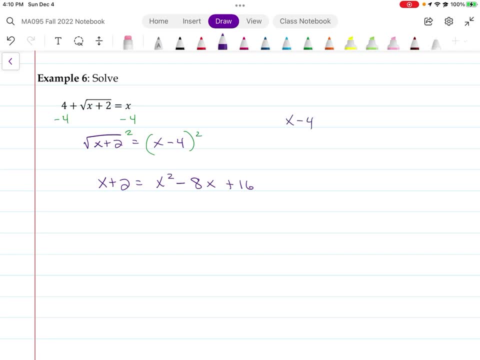 plus 16.. So remember, x minus four squared is x minus 4 times x minus 4 and if you know all of the perfect square binomial expansions which we talked about when we were doing special factors, you can just think through it and to get the x squared minus 8x plus 16.. 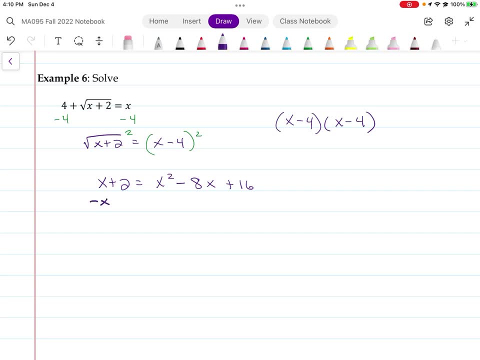 all right, moving on. all right. so i'm going to just subtract x and subtract 2 from both sides, so that i get 0 equals that and i'll have x squared minus 9x plus 14 equals 0. so now we can solve by factoring. this is how you solve quadratics: x minus 7 and x minus 2, so i get x equals 7. 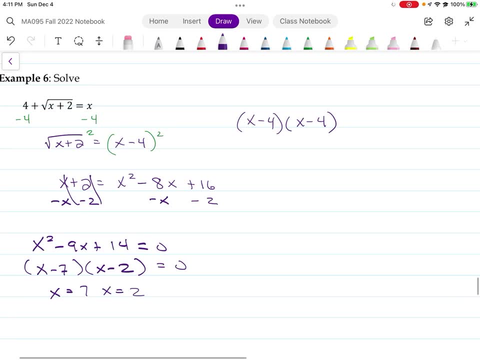 and x equals 2 and you can bet one of them is not going to be okay, so we're going to have to check. i'm going to erase this right here so i have room. so we're going to check over here. so, and check both. right, check both. so i'm going to check my x equals 7. 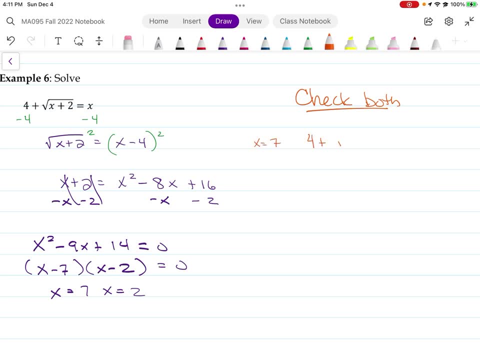 by plugging it in and i get 4 plus the square root of 7 plus 2 equals 7. so 4 plus the square root of 9 equals 7. so 4 plus 3 equals 7. that is true. so now let's check: x equals 2. this probably is not going to work, so we've got 4. 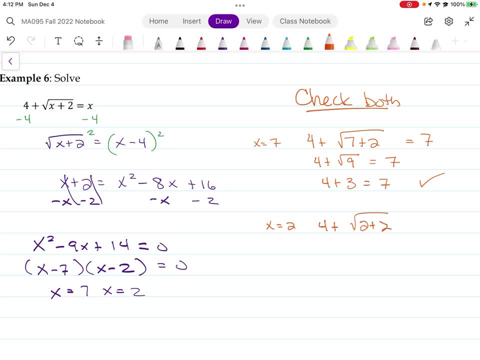 plus. plug in 2, 2 plus 2, fix that equals 2. so 4 plus the square root of 4 equals 2. 4 plus 2 equals 2. no, it does not okay. so instead of- instead of saying crossing it out, i should. 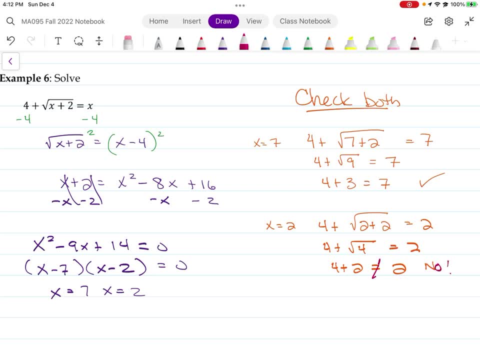 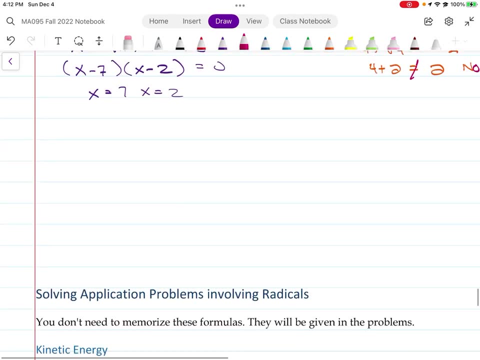 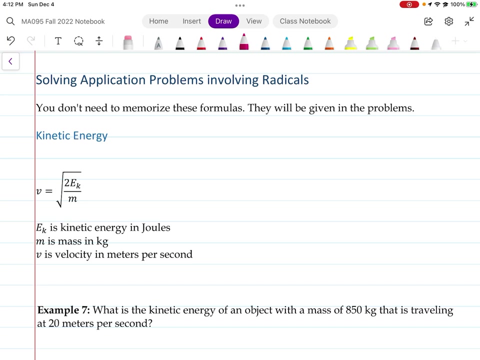 just say: does not equal, does not equal. so it's a no. all right, let's try another one. oh, actually we're moving on to applications. i've got a couple of applications here. you don't need to memorize these, they're going to be given in the problems. this is the equation for kinetic energy. 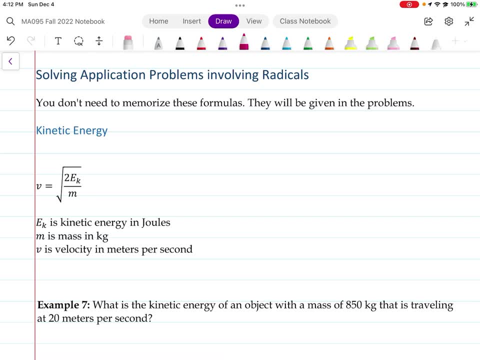 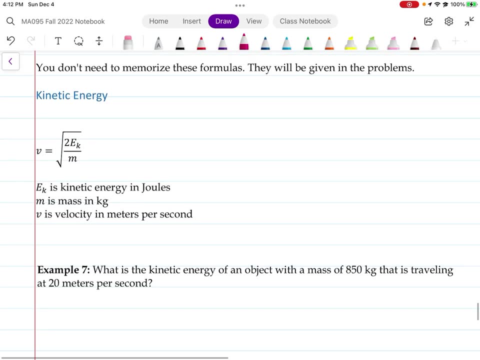 where v is velocity in meters per second and m is mass. e sub k is kinetic energy and it's measured in joules, all right. so what is the kinetic energy of an object with a mass? so they're giving us the mass. i'm going to write this down: mass equals 850 kilograms. 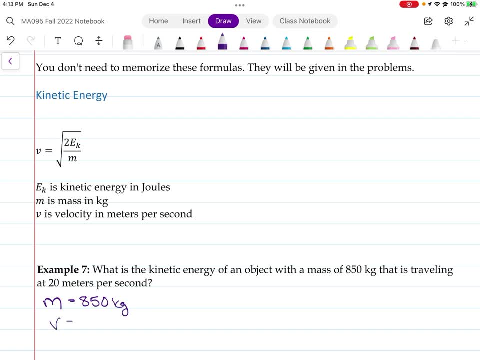 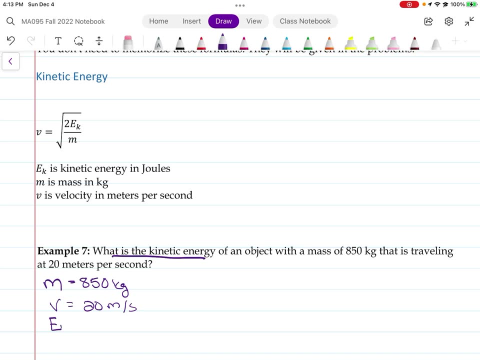 and it's moving 20 meters per second. that's velocity, 20 meters per second. and it wants to know what is the kinetic energy. well, that's e, sub k equals question mark. okay, so that's what i always do with word problems. now i don't have to look at it anymore. i've got all i need right here. 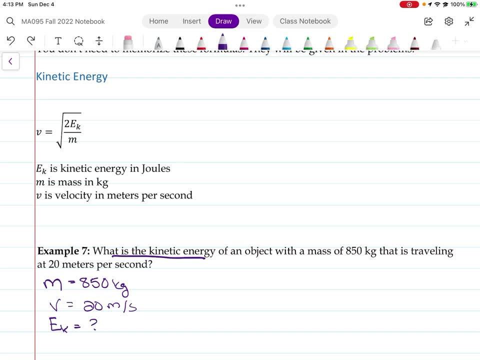 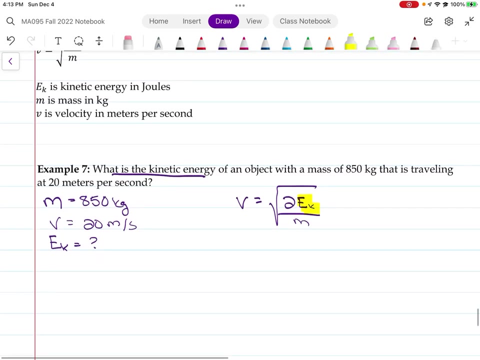 all right. so now we've got this formula that's: v equals the square root of 2 e sub k over m, and i am looking for e. so let's practice rearranging a formula without numbers in it. it's just a lot faster. so we're going to square both sides. 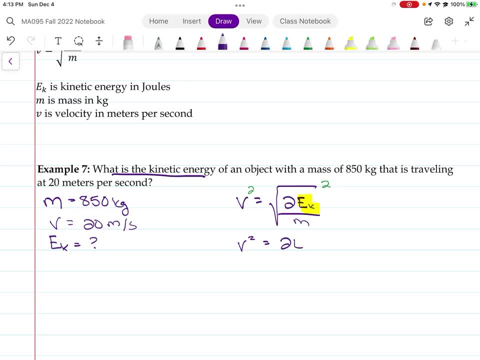 and i get. so i get v squared equals 2 e sub k over m. now, what well, i need to get the e. i'm going to keep highlighting it so we can think about what we're doing here. i'm going to multiply both sides by m. 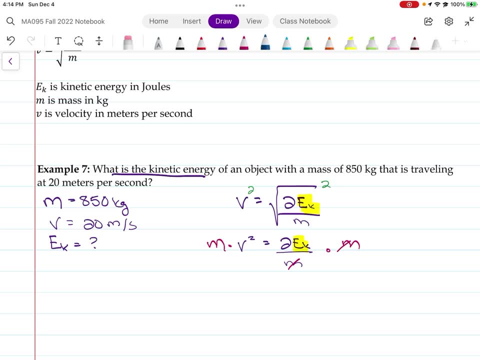 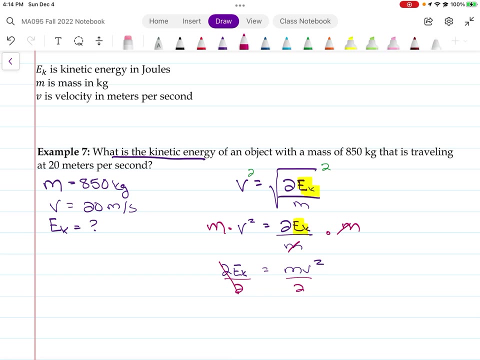 so they cancel out over here. and so now i've got um, i've got e, i'm going to switch sides. 2 e sub k equals mv squared, and now all i have to do is divide both sides by 2.. it's so much easier than rearranging with a. 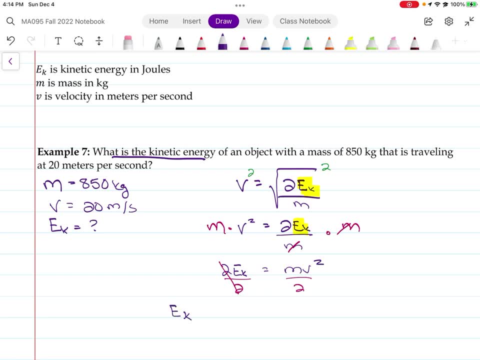 bunch of numbers in there. i, i think you might not, but, um, you could do it either way. you could plug in the numbers and then rearrange it. you're going to do the same things. so we've got ek equals mv squared over 2.. all right, so m is 850, 50 kilograms, and v is 20 meters per second, and we square that and that's. 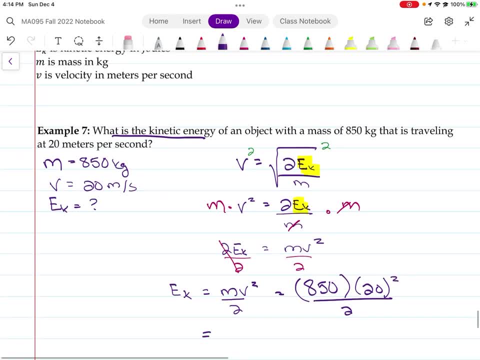 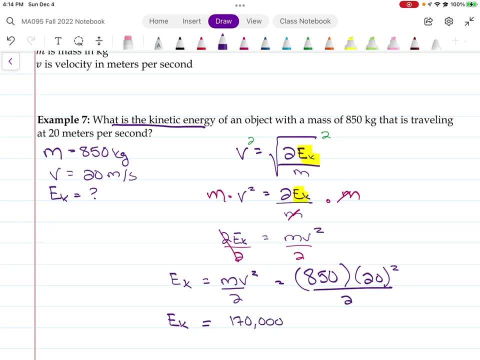 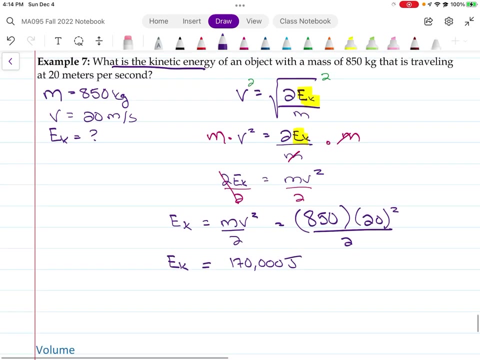 all over two, and when you put that in your calculator, you're going to get that the kinetic energy of this object is 170 000 joules, and that's why we use kilojoules a lot, because joules are tiny, all right. next is one with two. 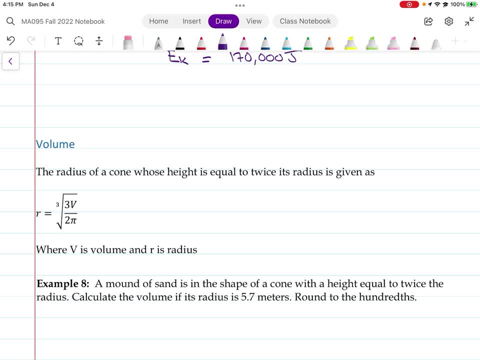 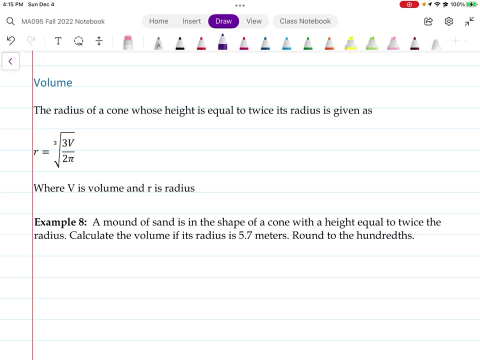 the volume. the radius of a cone whose height is equal to twice its radius is given here, where v is the volume and r is the radius. so amount of sand in the shape of a cone with a height equal to twice the radius is is given here. so we're supposed to calculate the volume, okay, so 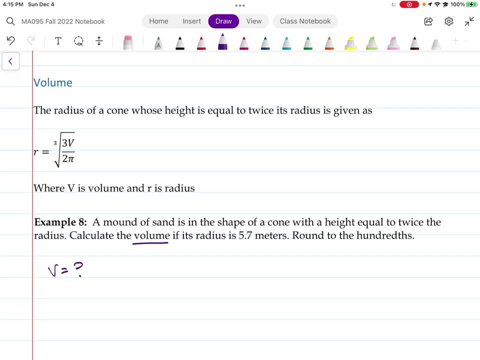 v equals question mark. calculate the volume if its radius is 5.7 meters. so we'll just say r equals 5.7 meters, and then we're supposed to round to the hundreds. okay, so there's a lot going on in that formula there, but there's only one variable that we're looking for. we're looking for v. it's on the. 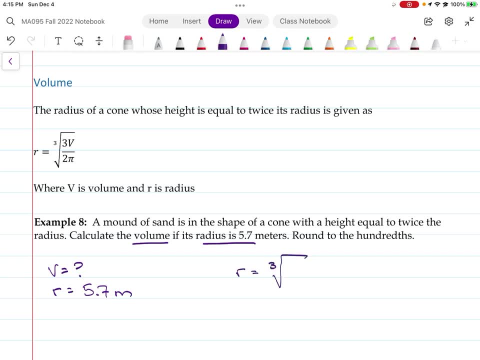 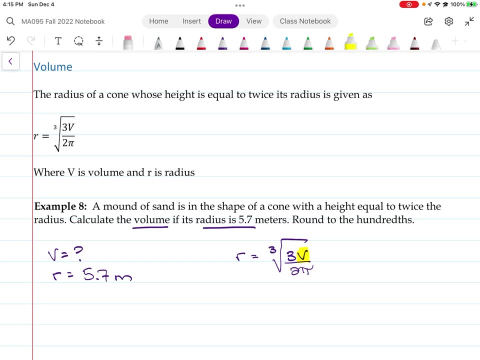 inside. so let's practice rearranging with just the variables. okay, so we're looking for the v. so what can we do to both sides to get rid of this cube root? hopefully, you see that we're going to cube both sides. cube a cube root and it goes away. so i've got. 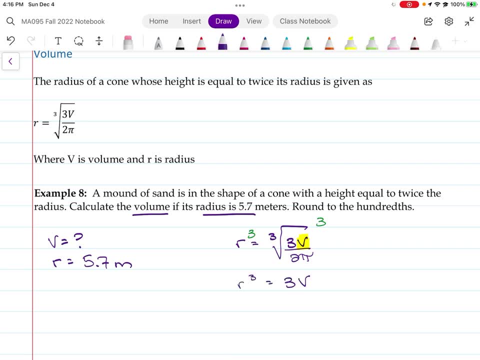 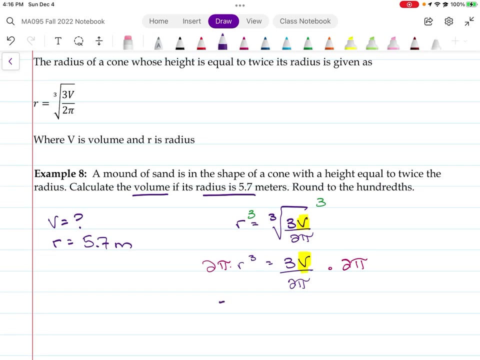 r cubed equals three v over two pi. All right, so you might be able to do this in one step, and that's fine, but I'm going to take two steps to do it and I'm going to multiply both sides by two pi and I get two pi r cubed equals. now this canceled out three v. Now I'm still looking for the v, so 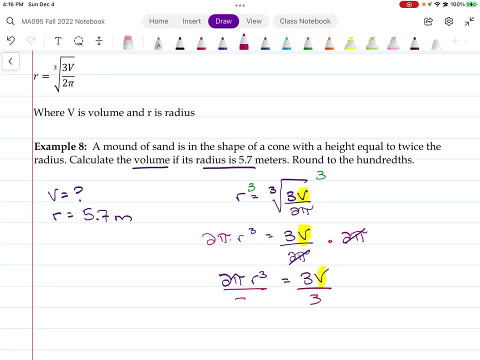 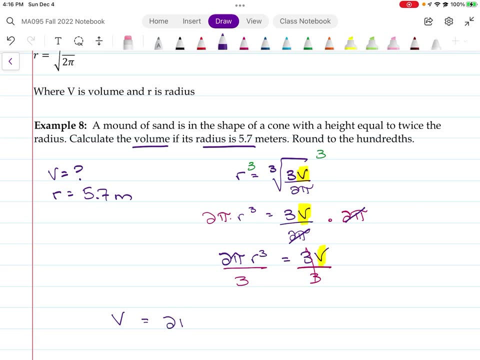 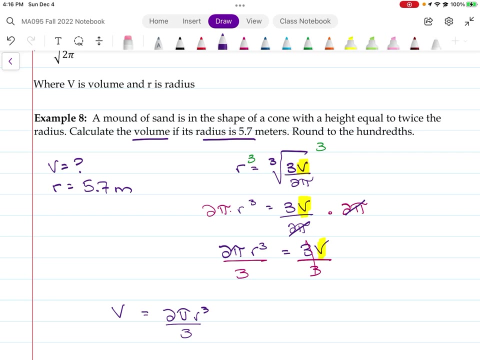 I've got to divide both sides by three, so I get divided by three. So I'm just going to rearrange this. so the v is first. I'm going to write it over here. v equals two pi r cubed over three, or you could say two-thirds pi r cubed, which is the equation for the volume of a cone. that specifically. 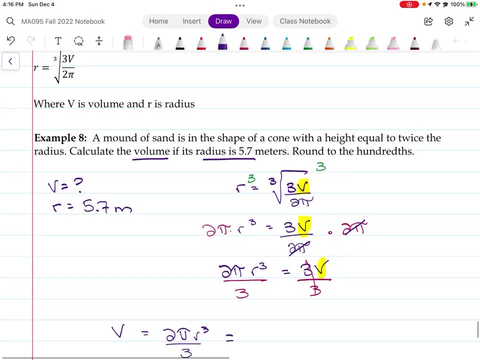 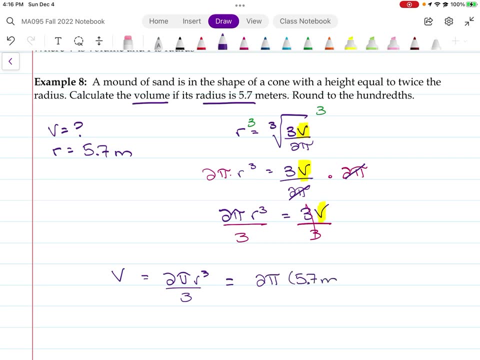 has. sorry, that specifically has a height twice its radius. All right, so we've got two pi 5.7 meters cubed. This time I put the unanimous it in because I want to see, I want you to see, what happens. so the meters is cubed, so that's.